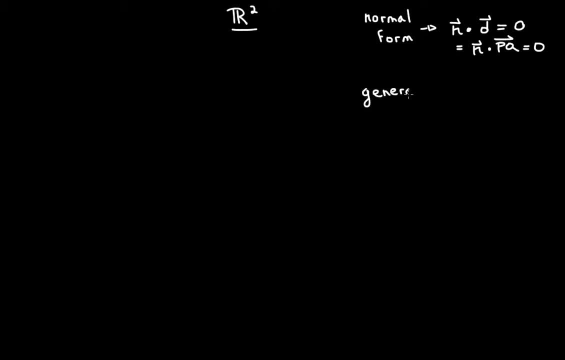 normal form And general and in general form. we talked about this in the previous video and if you haven't watched that video, then I would advise you to go back and watch it, because it's very important for you to understand what we will be doing today. So the general form is n sub. 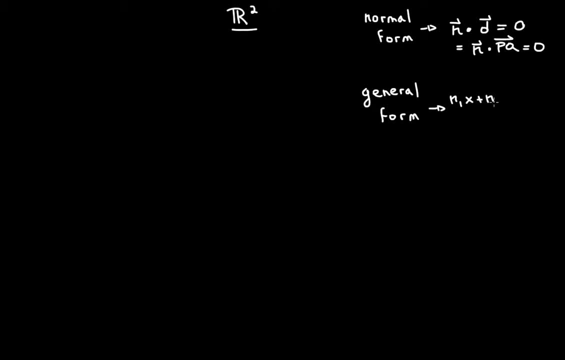 1 times x plus n sub 2 y, equal to some sort of number or constant k. So we have four different types of ways of expressing lines in R2.. We only know half of them In this video. we will learn the other two. 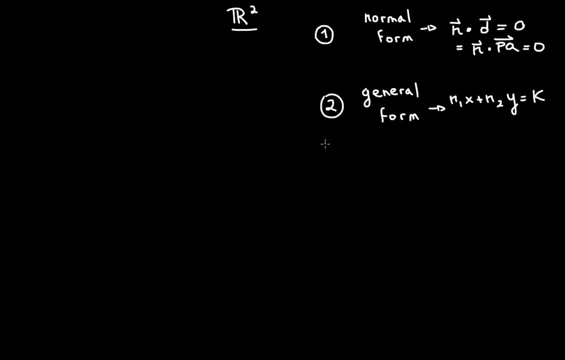 two, and both of them are, you know, really, really important. just like we started with a sketch for a normal form, let's try another sketch to understand what it means to be you know what the line, or the or or what the equation means, and when we say that, well, we are expressing it in terms of, you know, a vector. 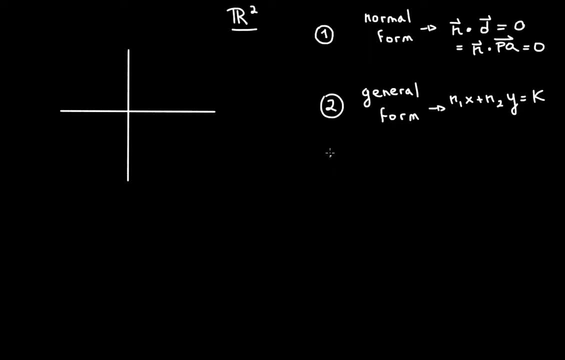 equation. so let's so, let's talk about that. so and just so you know, we don't know. let's just so you know. I don't want to spoil it for you. however, this is what we will be learning, first of all. the third equation will be the vector. 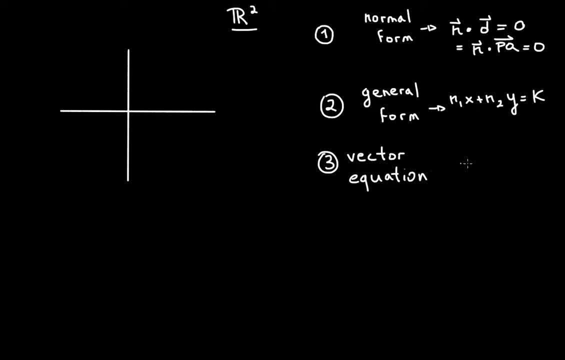 equation, and the fourth equation that we will learn will be, will be, and the parametric, para parametric equation, both of them equally important. so, for the vector equation, what we want to think about is: okay, imagine some sort of line, you know, let's say that we have a line here and let's say that we have a line. 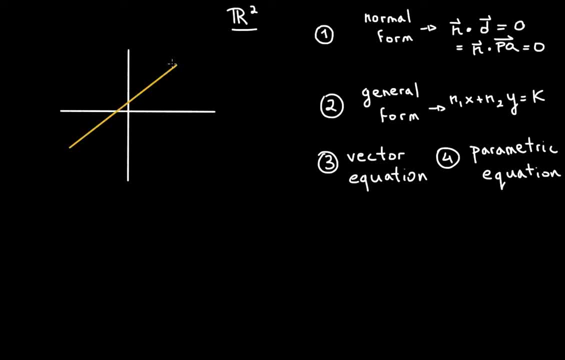 some arbitrary line limit, so maybe that's our arbitrary line. then, you know, for some reason we we want to look at other lines that are parallel to this. however, one way that we defined this line recall that we said, well, there must exist some sort of point right over here and let's call that p, and, and maybe this: 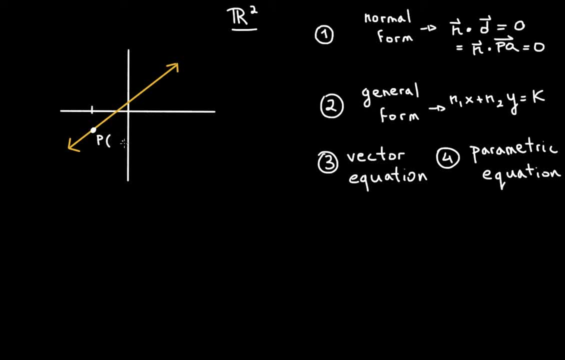 P is, you know, maybe, that's maybe. so you know this is defined by a and B. so you know this might be a and this y height might be b. and we said, well, we could have another point, p and q, which has coordinates x and y. so you know this would be x, so this would be so. so the x direction. 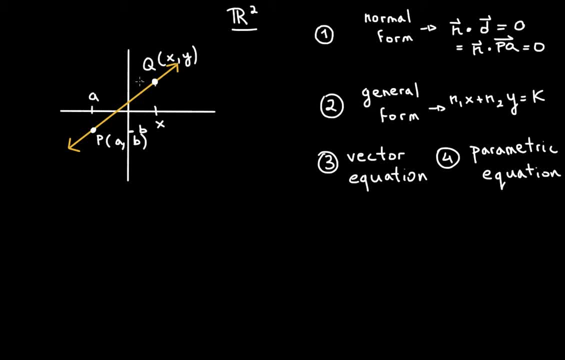 length would be x and then this would be y. so using this, we said that the vector p, so some you know, a vector that goes from what the vector, and the point p to point q. so this vector would be the following: p to q is a vector, so the final minus initial. so we have first we for the 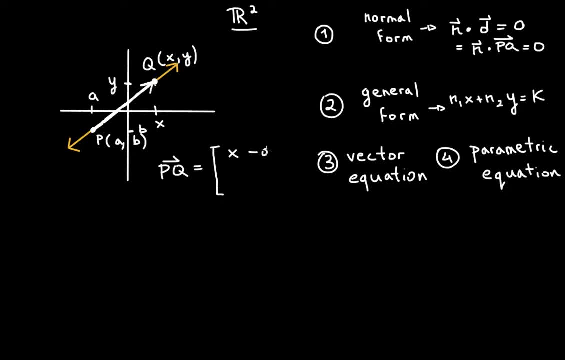 component. we have x's, so we have x minus a and then we have, uh, you know, y minus b, y minus b. so this is all the news for you. so, in so for vector equations, what we imagine is okay. you know, there are infinitely many other parallel vectors. 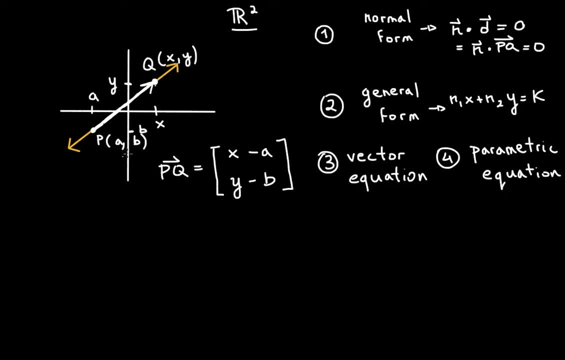 to pleasantÚ our vector PQ. So if I draw a vector that's this long and, you know, going in the same direction, and this would be parallel, If maybe that vector that's also parallel and this vector is also parallel. So I guess- and you know a good way to to write this- would be well, all of these or any. 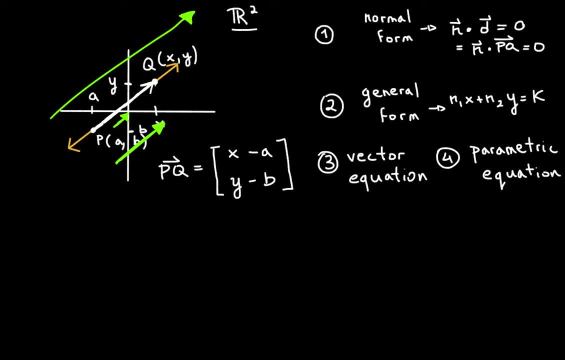 green vector could be scaled back to the size of this white one. All right, let me change the color, let me make it red, Let's make it red. So you give me any vector that's parallel to to our vector, or this red vector, PQ, Then what I can do is I can give you another vector which is parallel to this. 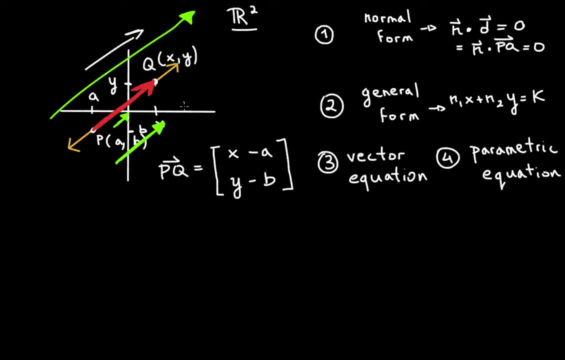 because there are infinitely many of them. One could be right over here and one could be right over here You. all you got to do is just translate it right over there and then it would be parallel, as long as it's going in the same direction, You know. and then, using that logic, 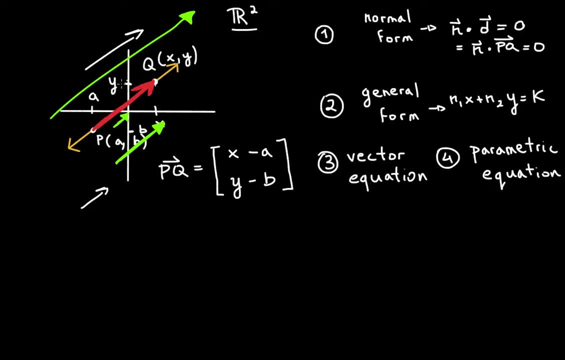 I could take any one of these and I could scale it to this size, to the red size, and those two vectors would be equal. So this green one, all it needs is to be scaled to be something bigger, and all this bigger green needs is to be scaled back to- well, you know, to a smaller vector, so that 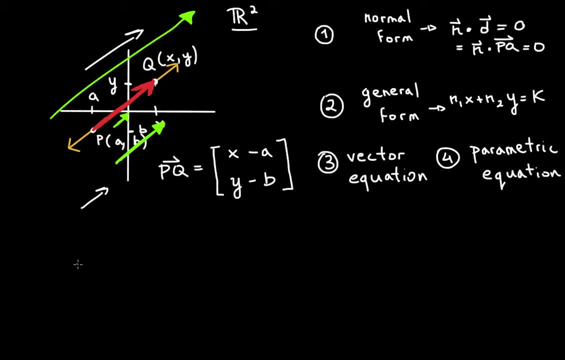 it can, so that it can mimic the red vector. So, using that logic, we can say that the red vector, which is PQ, is equal to. so, if, I, so, if, I, so, if, if, if the vector D is denoting any direction vector, that's, you know, in the same direction as our. 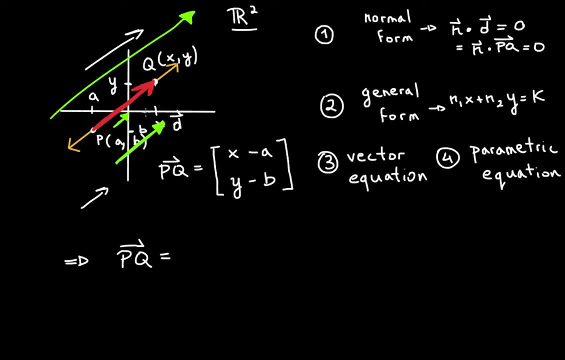 vector PQ. So you know, this is: this could be a vector D, This little one could be a vector D, This bigger one could be a vector D, This white one would be a vector D, So any arbitrary vector that's parallel to that, so it's going in the same direction as our red vector. Then if, if you give me a vector, 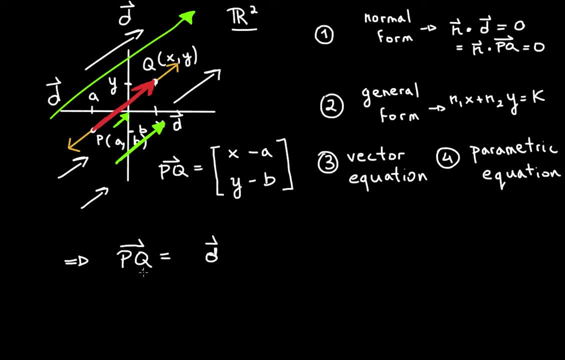 D, all I need it to be equal to the red vector. So here I will just give it a little outline that I will give you an idea of what that looks like. So I will just say that the red vector is some sort of scalar, And let me call that scalar T. So we would have T, and so you know. 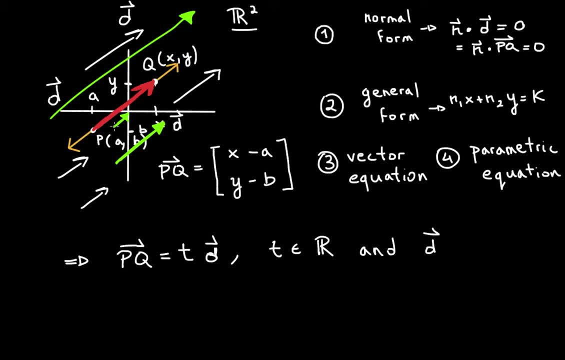 d is defined. we don't know the dimension. you know whether this was arbitrary or this bigger one is arbitrary, and since it could be any number, we we've just generalized it. so the first component would be d sub 1. second component would be d sub 2. so, using this logic, what we can say is that well, 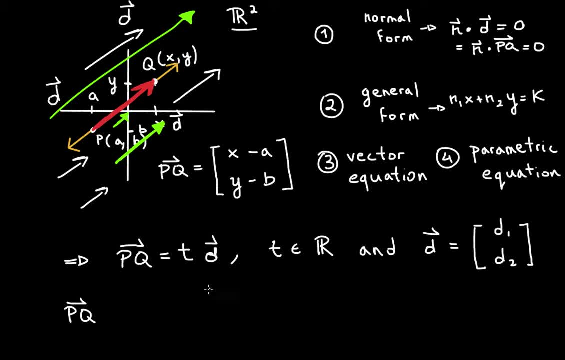 pq is equal to what, pq is equal to that, so pq is equal to that, all all that material. so x minus a and then y minus b. so therefore, since that's pq, so and pq is equal to that, therefore this must be equal to that. so this is equal to t times times d 1 and d 2. so where did i get this? that's the. 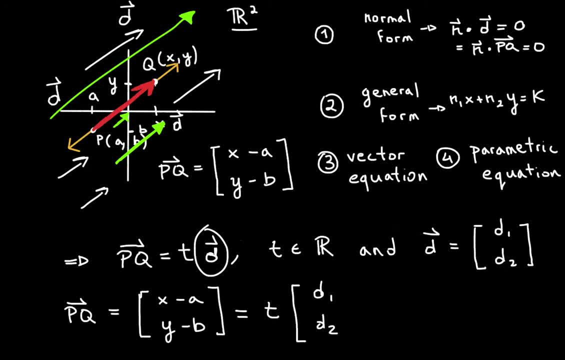 d vector, which i defined right over there. so so, and then that, however, we we now we know what scalar multivariate multiplication is, so the t can go inside. so this would be equal to t d 1 and then t d 2. let me box this for you, because this is called a vector equation. let me box this for you. 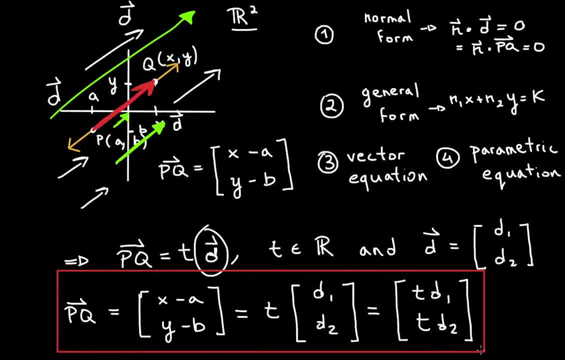 we will be doing some examples, um if and for for these, so that you can perfectly understand how how these work. and once you understand what vector equations is, you can from. from there, we can create parametric equations, just like. just like. after understanding normal form we created, let me so, after learning about normal. 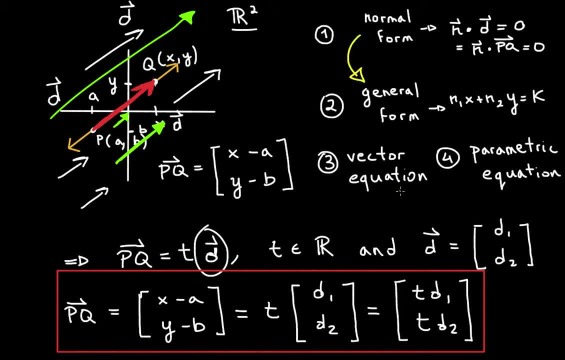 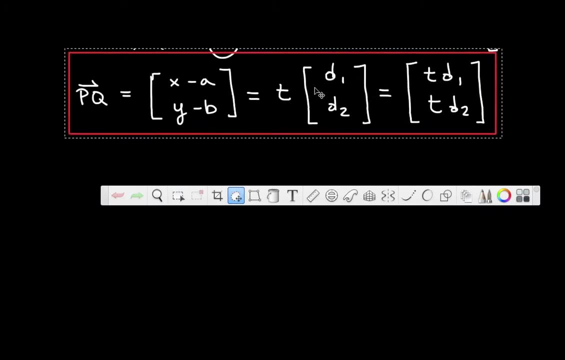 form, we could create the general format. after learning about vector equation, you can create the parametric equation. so so let me select this and let's go to a new slide. so let me just select this so we can go to a new slide. there we go. so from this, we call this the vector equation. we can create the parametric equations. 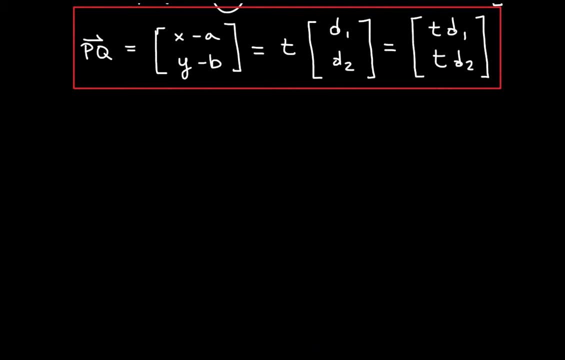 so we, how do we do that? we only focus on this portion and in this portion. so this is an equality. so i can basically say: well, this is equal to that. so what i mean is: if this is a and that's b equal to c, equal to d, what i'm saying is: well, since a is equal to b and b is equal to c and c, 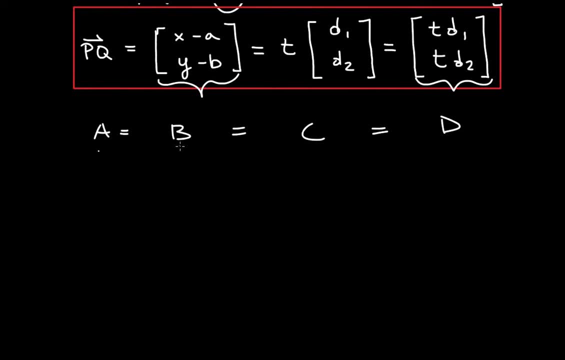 is equal to d, then therefore we can create the parametric equations, we can create the parametric. Therefore, b is equal to d. That's just normal logic. So you know, through that logic I'm going to equate x minus a. 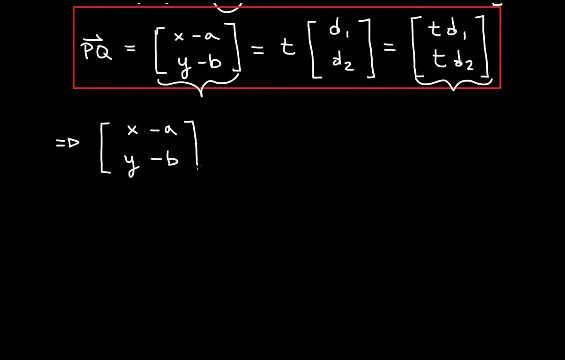 then y minus b is equal to t d1 and then t d2.. So now, something that we will learn in just a few videos is the systems of linear equations. However, for now, you can just take my word in, wherein I tell you that these two are equal. 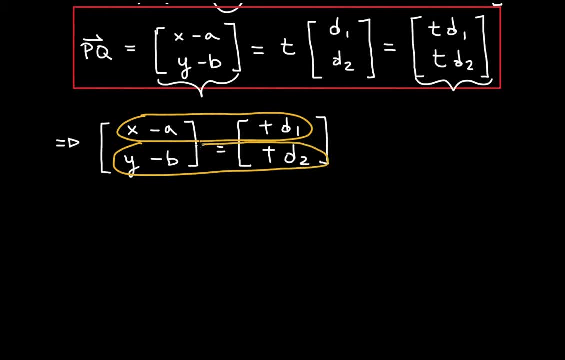 You can say that they're equal. and these two are equal as well. So the set of parametric equations that you would have would be: x minus a equals to t d1.. And then you can just take my word in, wherein I tell you that these two are equal. 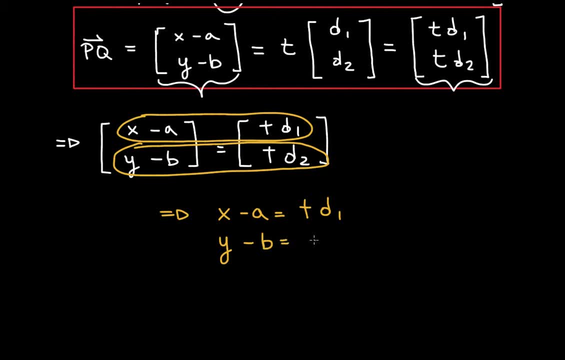 So the set of parametric equations that you would have would be: x minus a equals to t d1.. And then bottom one would be y minus b equals to t d2.. Now we don't. this looks ugly, So we want to isolate for x and y. 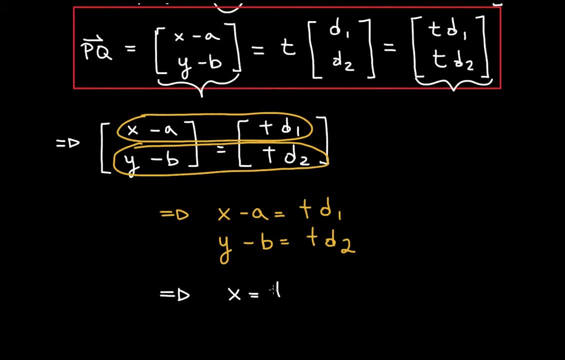 So, therefore, our x is equal to t d1 plus a, And then y is equal to t d2 plus b. So, once we understand this, we are good to go because, ladies and gentlemen, we have. we have. let me, I'm trying to box this for you. 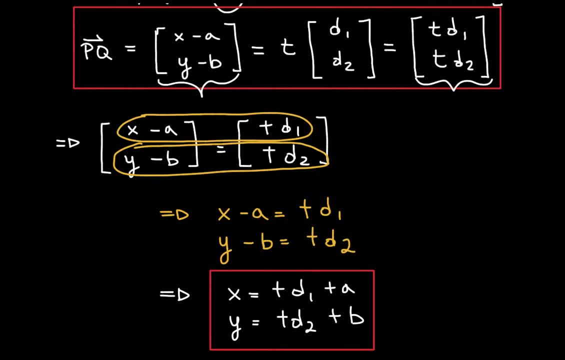 There we go. We have two, well, the set of parametric equations of line L. So these are parametric, parametric equations And the top ones are vector. So this would be a vector equation. I believe it's only fair to. 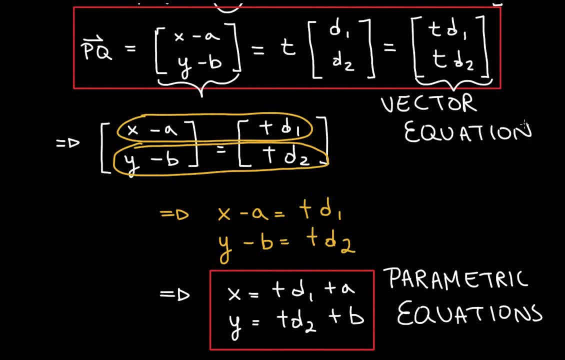 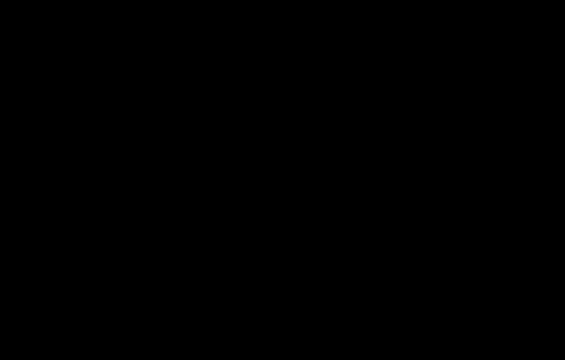 to end this video with with an example. So let's give it a shot, So let's create a new slide, And this would be, I guess, our second example, because in the previous video I showed you how to create normal and general forms. 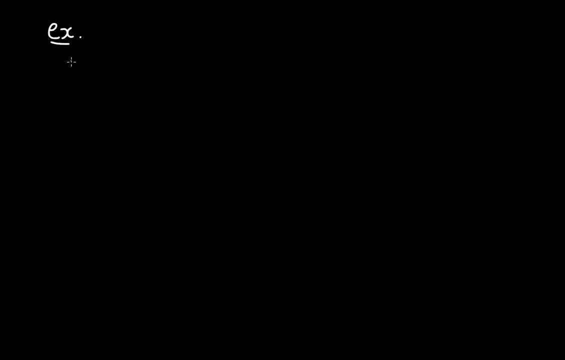 So now let's learn about how we do it with vector and parametric. So they might ask: you find a vector, So find a vector equation, Vector equation, Vector equation and and parametric equation. Or I guess I should put vector and parametric together so I don't need to write it twice. 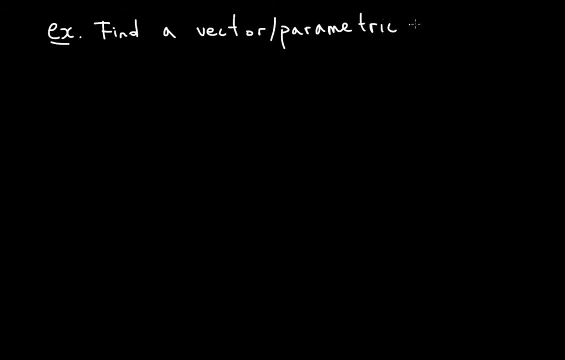 Parametric equation or S, depends on which one you're reading: of line L, of line L Which, which goes through, which passes through the point which, which goes through the point P, which is equal to 2, negative 5, the set of coordinates. 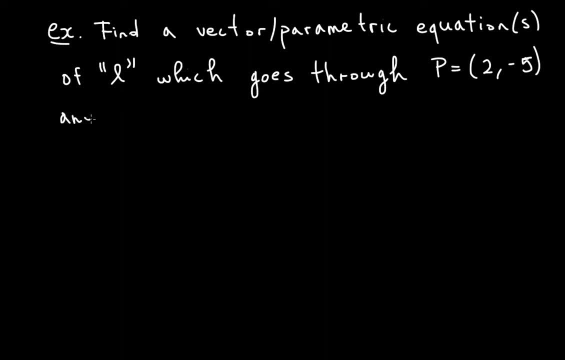 And in the direction, and in the direction of of the vector D, which is equal to 1, 3.. Now, the two matrixes, The main pieces of information that they give you, are this point, this one. They give you P and they also give you D. 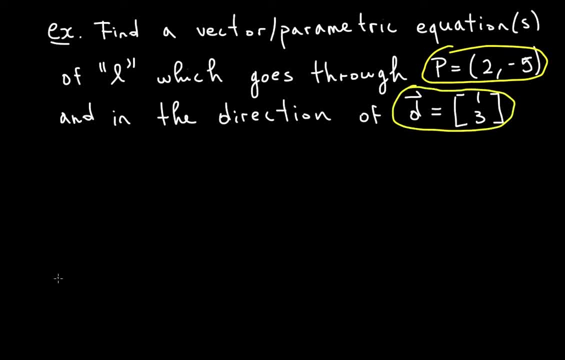 So hopefully you haven't forgotten what the vector equation looks like. The vector equation, just just in case you forgot, would would be: you know, PQ equals to X minus A, X minus A, And then Y minus B, which is in return equal to T. 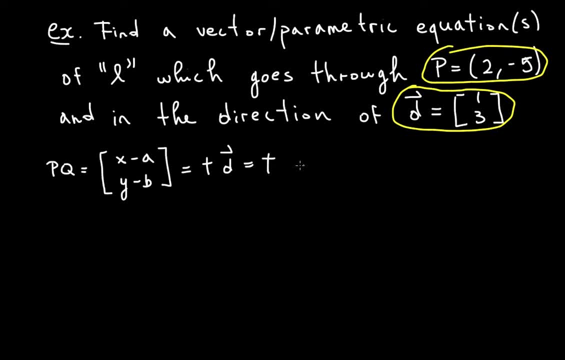 Then times the vector D and which is equal to T, And we defined D to be D sub 1 and D sub 2.. So again, we only look at this and this for for our purposes. So from this we say that, well then, this will be your A. 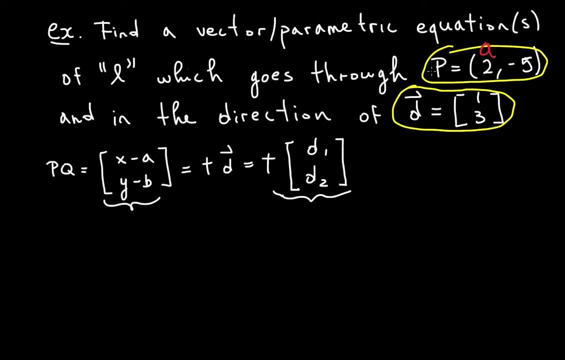 So you say this will be my A, So again, X and Y. you normally keep it general. In the previous video I, I, I showed you that that's not really necessary. It depends on What you said and you know. you can draw a sketch and you you can do what I did in the previous video. 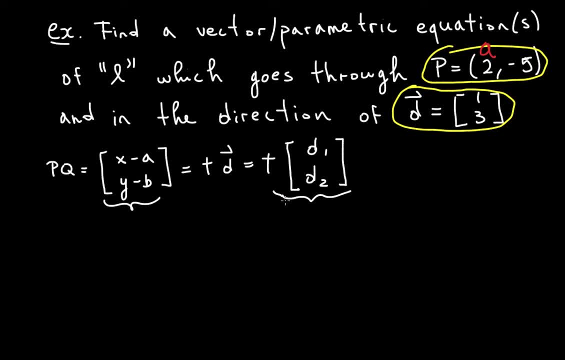 However, normally you want to have X and Y to be the unknown values. So so, using that, we know that this will be equal to what? So this will be X minus 2. Because that's our A and we say that's our B. 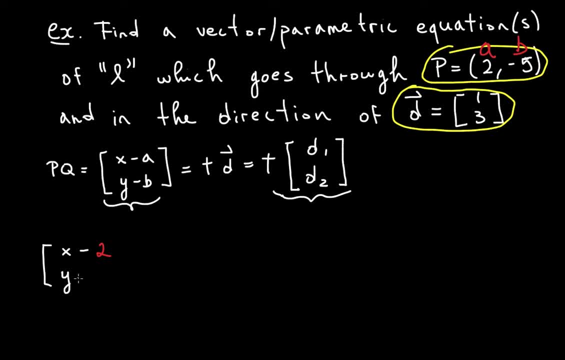 A, B are the values that they give you, And then Y. So minus, Minus, Minus will make a plus, So that will be plus 5.. So this this vector will be equal to T times the D vector. 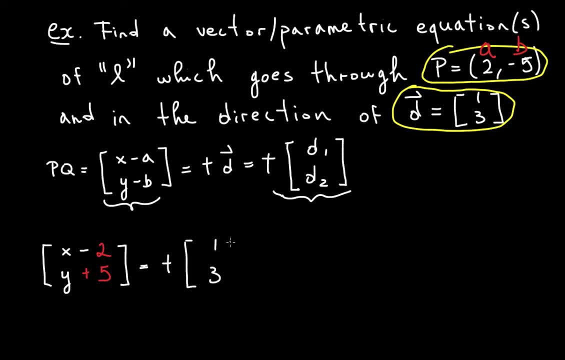 And the D vector is given, So it will be 1, 3.. So this will be your vector equation, And I guess you could put it in terms of this, and you can make this equal to PQ. However, you know, I, I, I have faith in you that you can do that on your own.